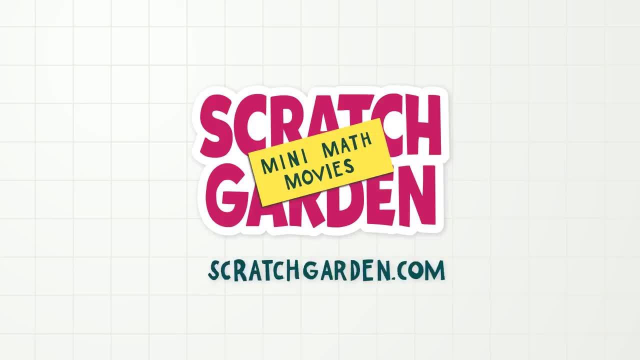 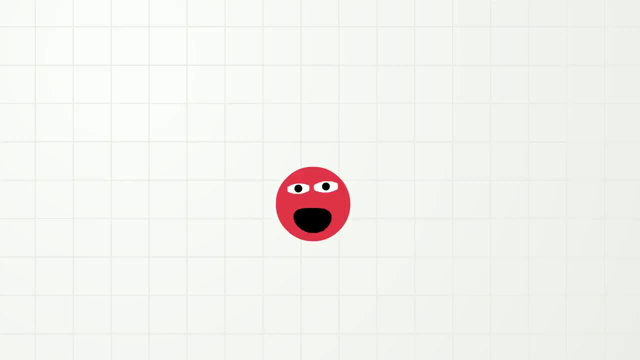 Oh, hi everybody. Today I am going to talk to you about numbers And composing and decomposing numbers, And maybe even apples. I really like apples. So composing is a large word Composing- And it's what happens when little numbers come together to make a bigger number. And 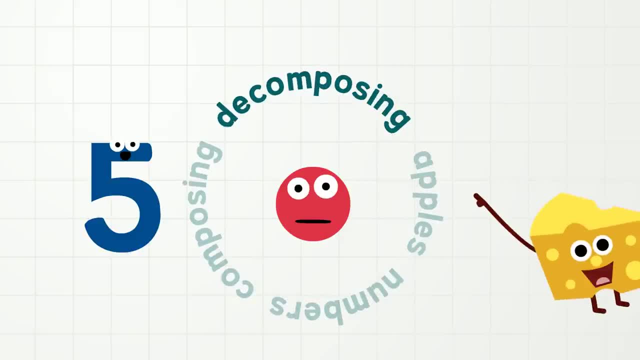 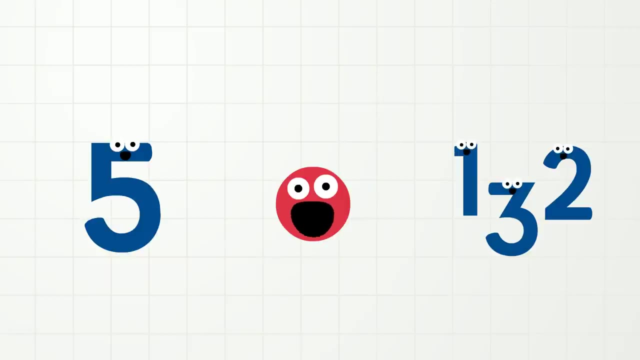 decomposing is an even larger word, Decomposing- And that is what happens when a bigger number is taken apart into little numbers. And there are many, many, many different ways to put numbers together and take them apart. I will show you with an example. Here we have the 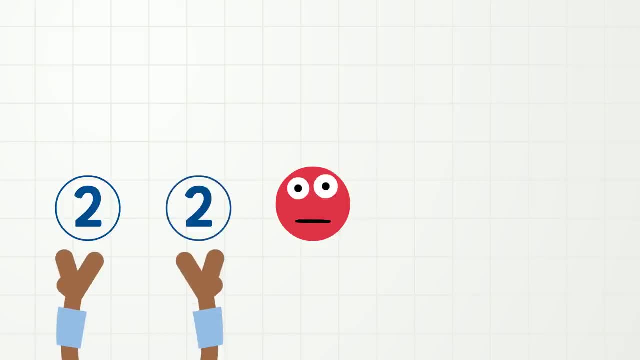 number two And there is another number two. What happens if you put two and two together? That's right, You get four, Four. This two and this two came together and made the number four. So four is made up of two and two, Which. 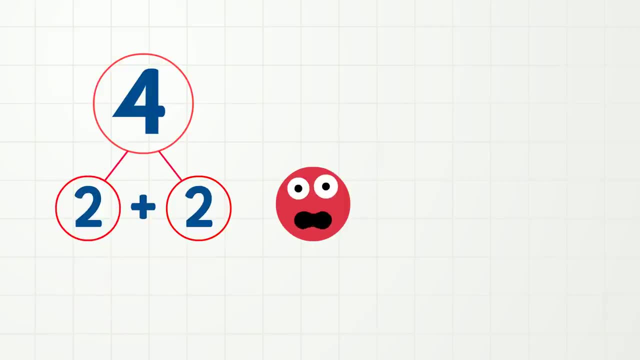 means four can be taken apart into two and two. Wow, We can put together and take apart the number four with totally different numbers. No, it's true. Watch, Here we have the number three And here we have the number one. What happens if you put? 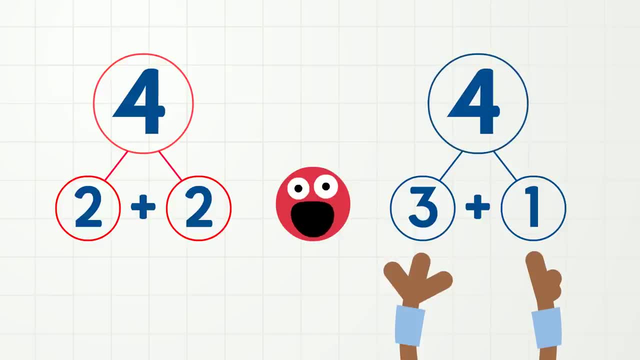 three and one together, That's right, You get four, Four. The three and the one came together and made the number four. So four is made up of three and one, Which means that four can be taken apart into three and one. WOW, So there are at least two different ways. 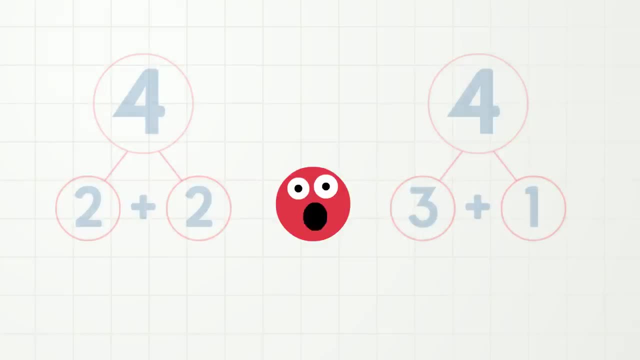 to put together and to take apart the number three and one. And if you look carefully you can see that the number three and one are the same number in number three and one, So it's apart the number 4.. Okay, you are doing such a good job listening. you can now watch a movie. 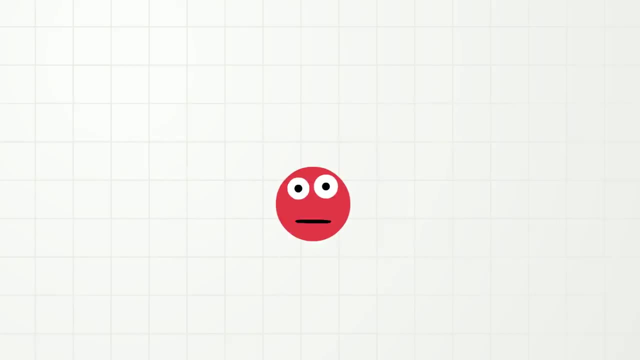 Okay, that's enough. This may be easier to explain if we have something to help us. Ah, I know apples. I said apples. Okay, look, we have one, two, three, four apples And we can take them apart or they can move. so we have two apples here and two apples. 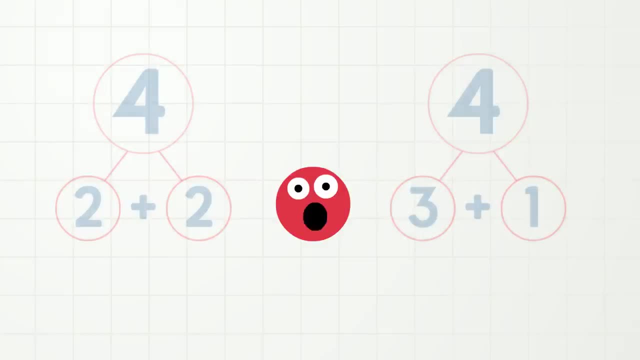 to put together, apart the number 4.. Okay, you are doing such a good job listening, you can now watch a movie. Okay, that's enough. This may be easier to explain if we have something to help us. Ah, I know apples. 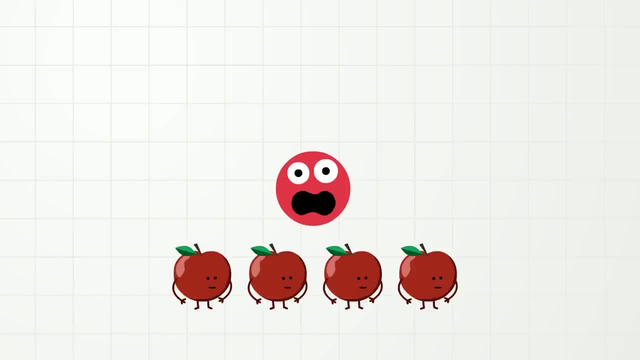 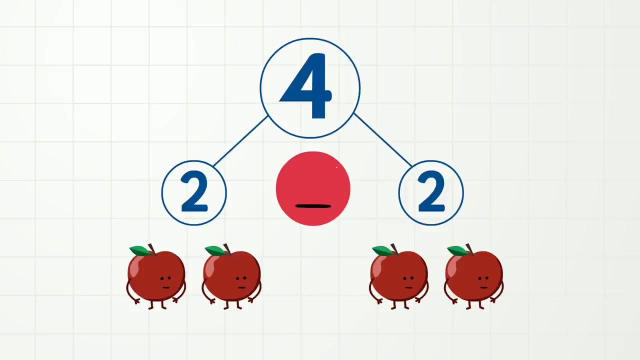 I said: apples. Okay, look, we have one, two, three, four apples And we can take them apart or they can move. so we have two apples here and two apples there, But we still have four apples. And what happens if one apple moves? 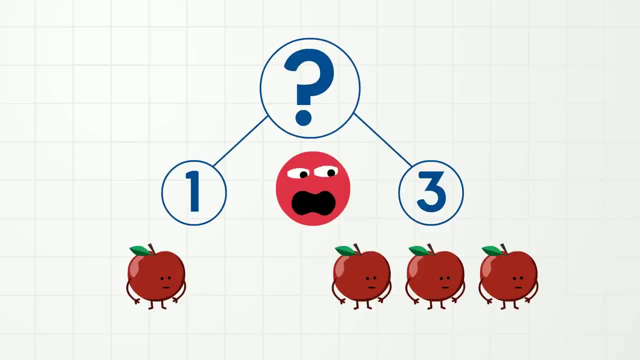 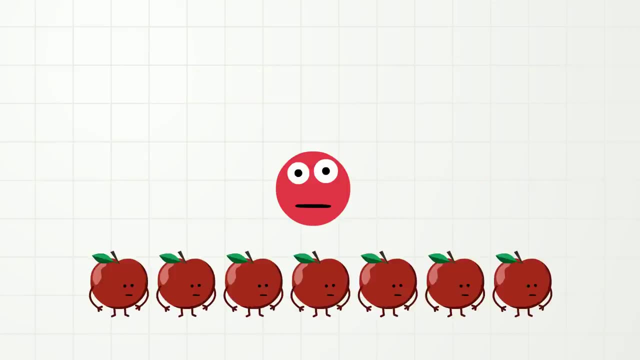 Well then, we have one apple here and three apples there, But we still have four apples, Apples. Okay, let us start again with some more apples. Now we have one, two, three, four, five, six, seven, eight, nine, ten, eleven, twelve. 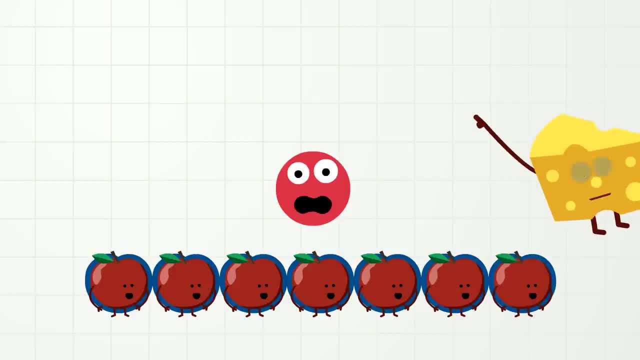 change six, seven apples, Apples. Let's see how we can take apart and put together these seven apples. Maybe we should use something to help us organize them. Oh, I know how about funny hats? Hah, Now let's have all of the apples with yellow hats go over here and all of the apples with 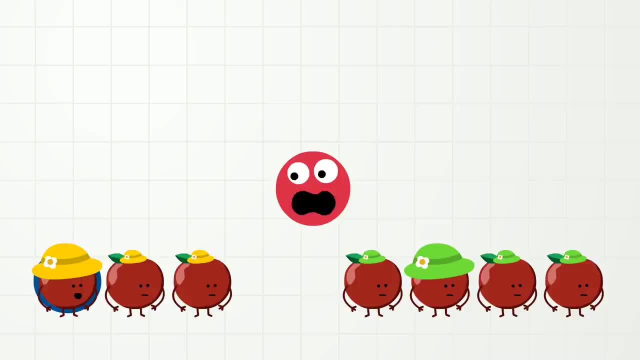 green hats go over there. Now have only one, two, three, four, five, six, seven, eight, nine, ten, eleven, eleven, twenty, thirty. Mmm. Well, that's Pass wollen. One, two, three, four apples with green hats. 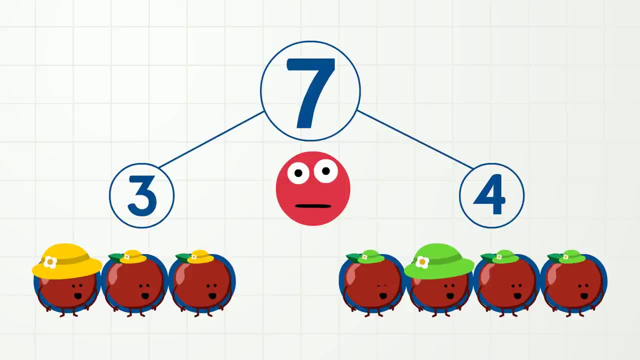 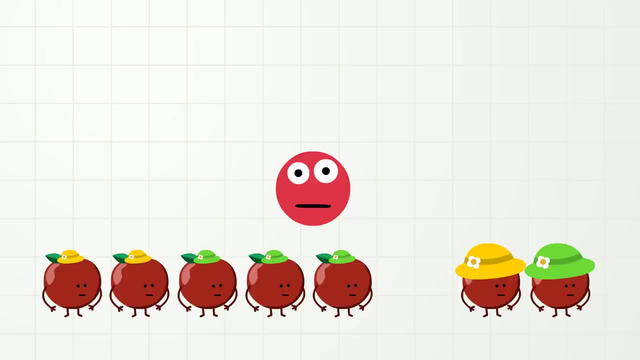 Add them together and we have seven apples. So the numbers three and four make the number seven. Now let's have all of the apples with little hats go here and all of the apples with big hats go over there. So now we have one, two, three, four, five apples with little hats and one, two apples. 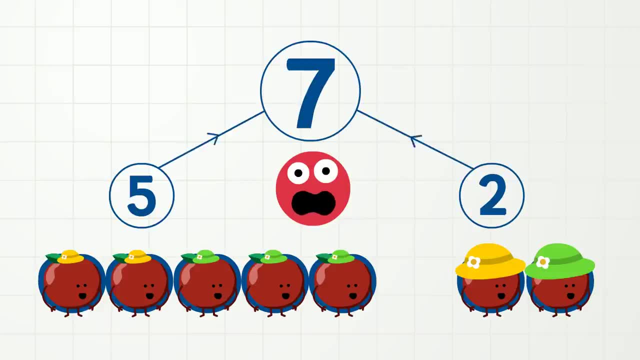 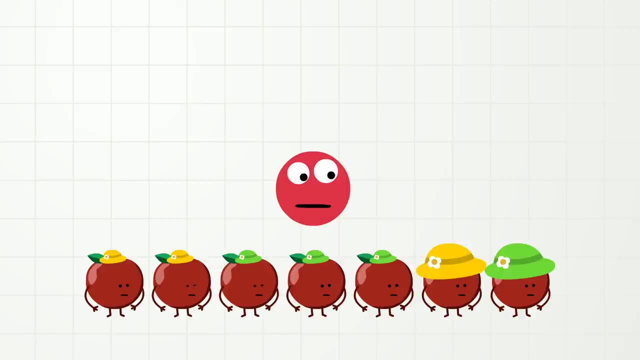 with big hats. Add them together and we have seven apples. So the numbers five and two also make the number seven. Wow, Seven. Okay, one more. How about all the apples that have a bite out of them go over here and all of the…. 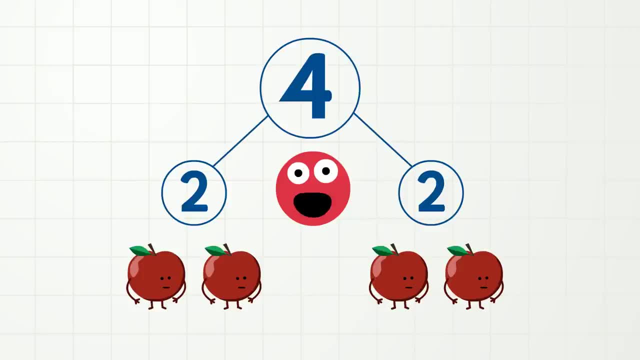 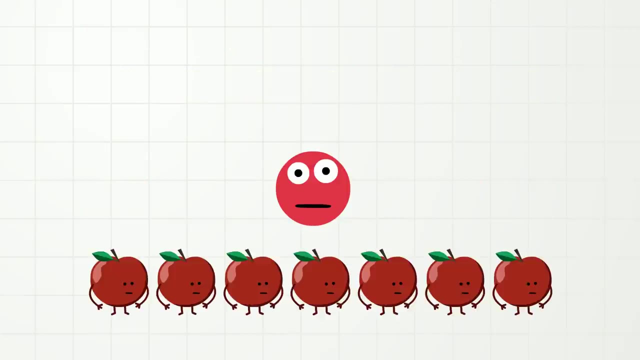 there, But we still have four apples. And what happens if one apple moves? Well then, we have one apple here and three apples there, But we still have four apples, Apples. Okay, let us start again with some more apples. 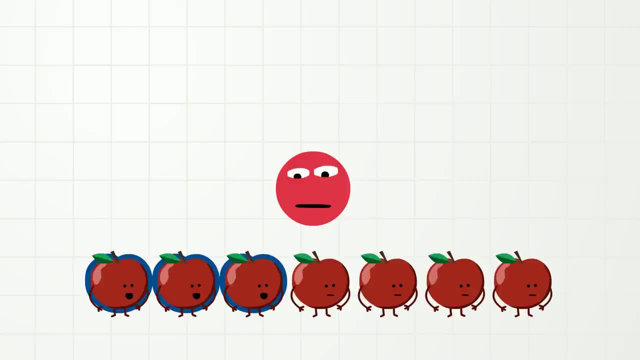 Now we have one, two, three, four, five, six, seven, eight, nine, ten, eleven, twelve, twenty Six, seven apples, Apples. Let's see how we can take apart and put together these seven apples. 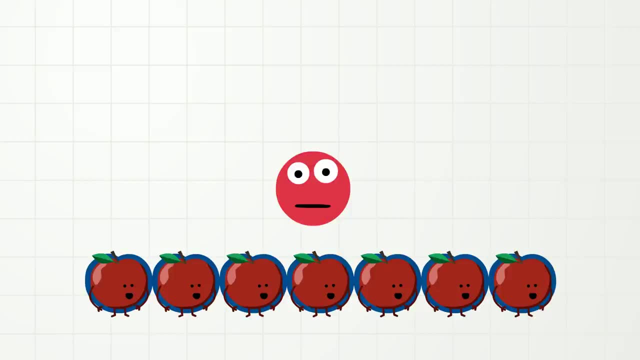 Maybe we should use something to help us organize them. Hmm, oh, I know how about funny hats? Ha, Now let's have all of the apples with yellow hats go over here and all of the apples with green hats go over there. 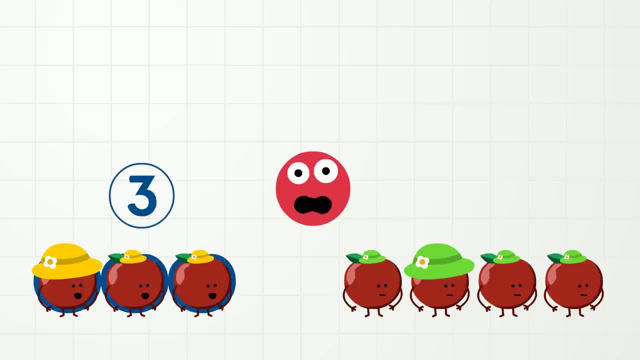 So now we have one, two, three apples with yellow hats And one, two, three, four apples with green hats. Add them together and we have seven apples. So the numbers three and four make the number seven Seven. Now let's have all of the apples with little hats. go here and all of the apples. 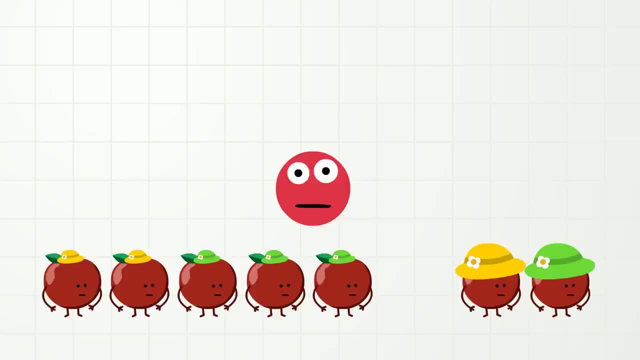 with big hats go over there. So now we have one, two, three, four, five apples with little hats, one, two apples with big hats. Add them together and we have seven apples. So the numbers five and two also make the number seven. Wow, Seven. Okay, one more. How about all the apples that? 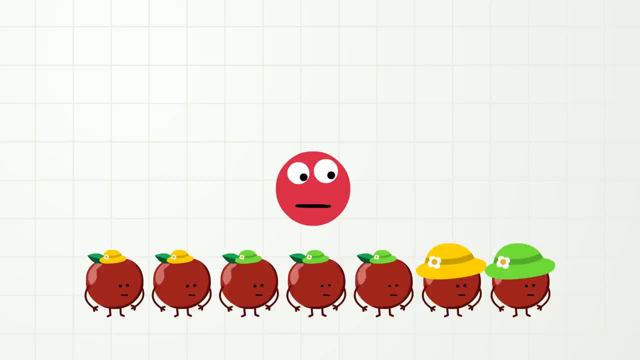 have a bite out of them, go over here. and all of the What's that? None of the apples have a bite. Oh well, we have to fix that. As I was saying, all of the apples with bites go over here. 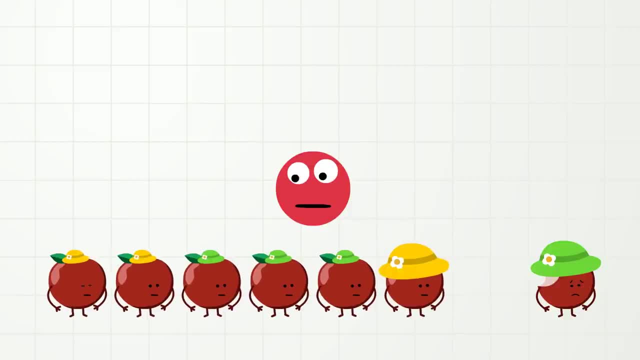 and all of the apples without bites go over there. So now we have one apple with a bite and one, two, three, four, five, six apples with no bites. Add them together and we have seven apples. So the numbers one and six also make the number seven. 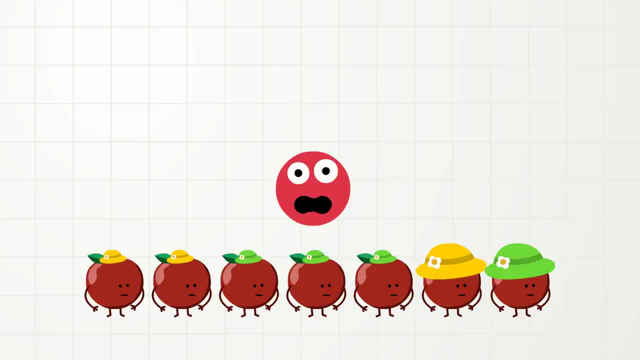 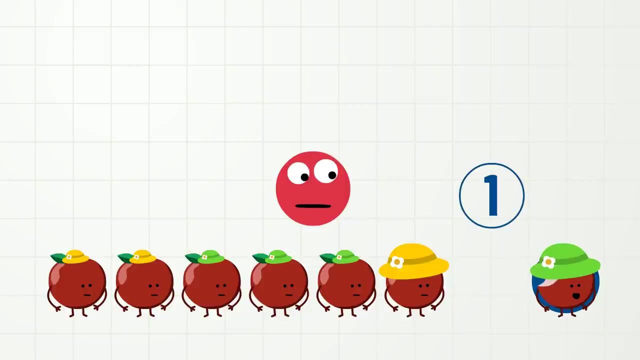 What's that? None of the apples have a bite. Oh well, we have to fix that. As I was saying, all of the apples with bites go over here and all of the apples without bites go over there. So now we have one apple with a bite and one, two, three, four, five, six apples with. 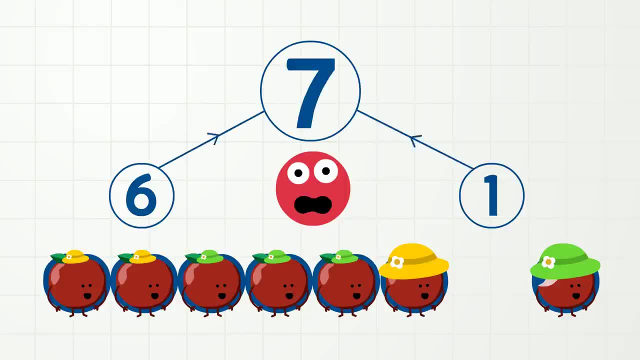 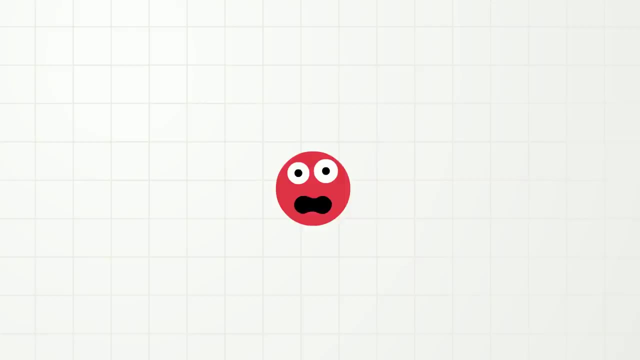 no bites. Add them together and we have seven apples. So the numbers one and six make the number seven. Also make the number seven: Seven. Okay, let's take a break and watch a movie. Okay, that's enough. Last one with even more apples, but this time no funny hats. 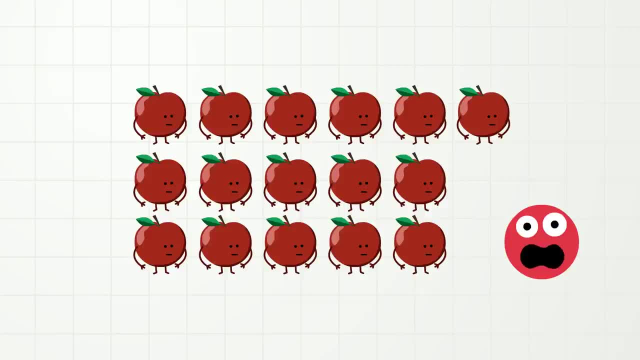 Wow, so many apples. How many? Let's count: One, two, three, four, five, six, seven, eight, nine, ten, eleven, twelve, thirteen, sixteen, seventeen, eighteen, nineteen, twenty, twenty, twenty, twenty, twenty, twenty twenty. 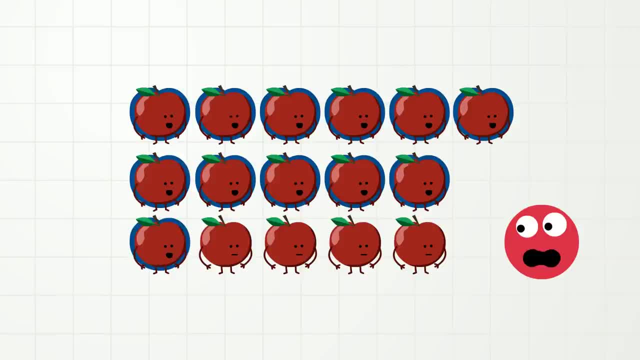 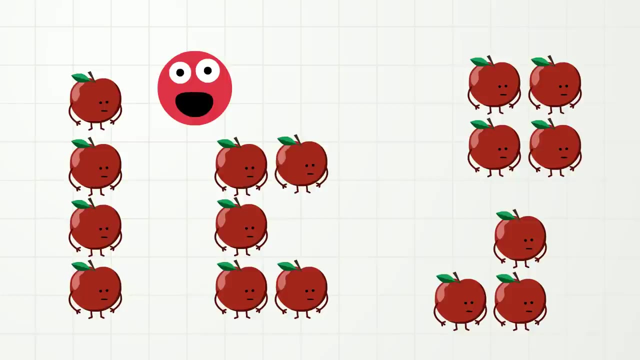 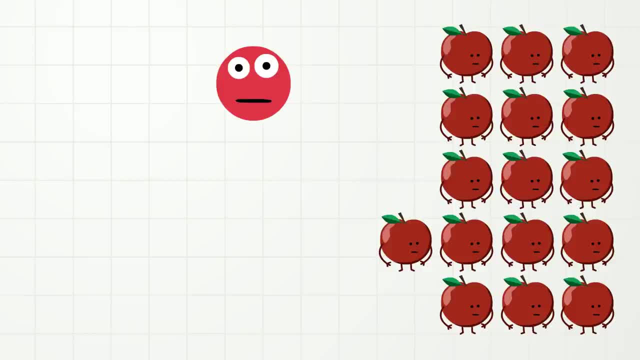 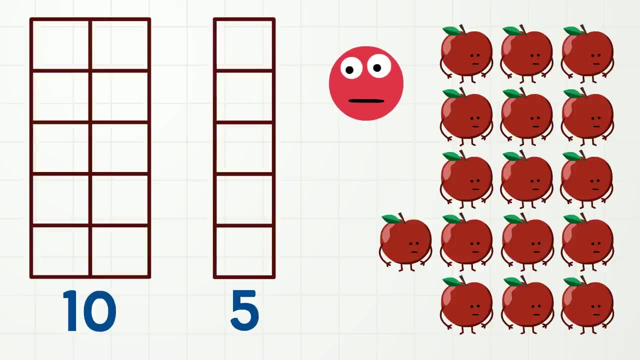 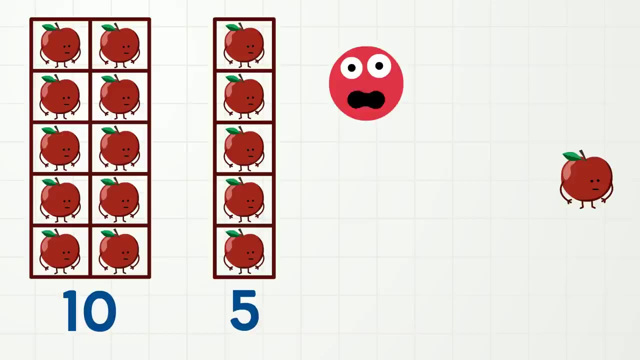 or take apart the 16 apples. Let's try some. Sometimes, when we are thinking about numbers, it can be easier to think about the numbers 10 and 5. When doing the 30-day. So if ten apples go here and five apples go there, how many apples do we have left? 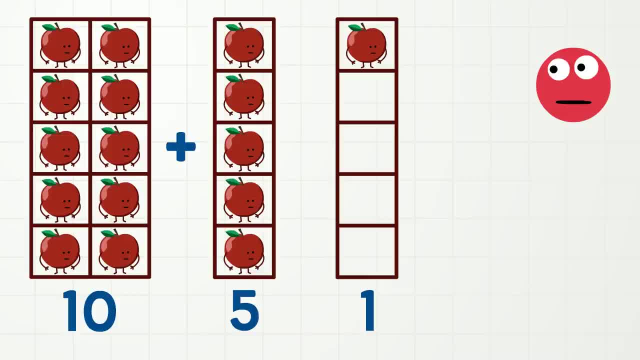 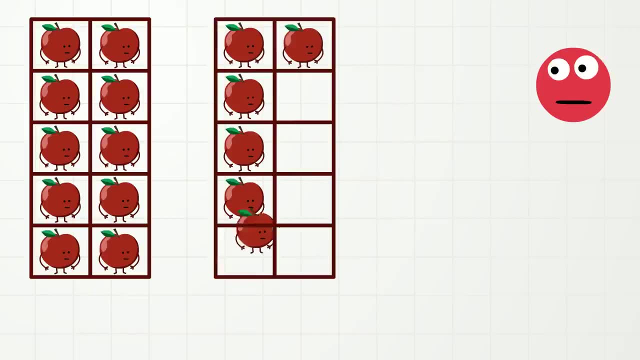 That's right. one, Ten plus five plus one is sixteen. So the number sixteen can be made up of the numbers ten and five and one. Cool, Let's try again. apples move. Oh wow, now we have one, two, three, four, five, six, seven, eight. apples over here. 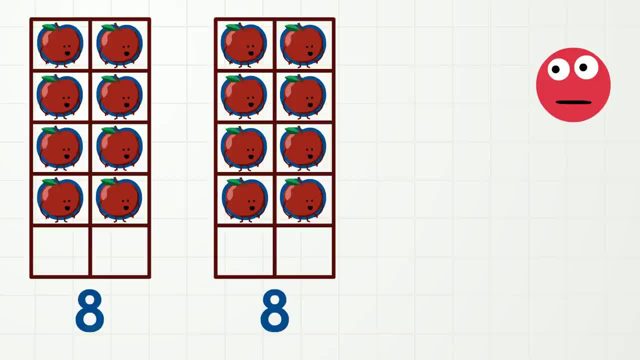 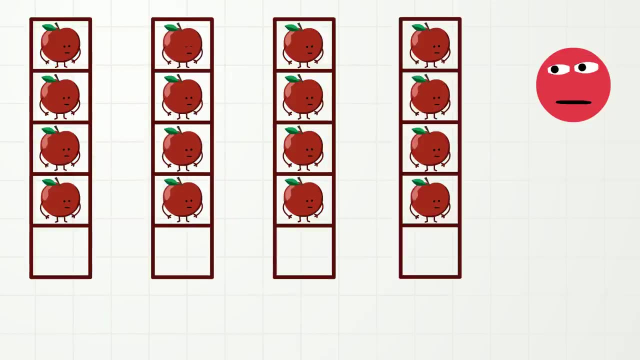 and the same number of apples over there. Eight plus eight is sixteen, So the number sixteen can also be made up of the numbers eight and eight. OK, one last time. move apples. Oh, cool, Now we have one, two, three, four apples here and the same number four apples here. 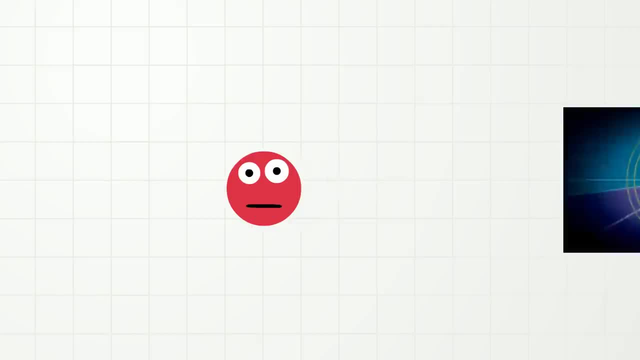 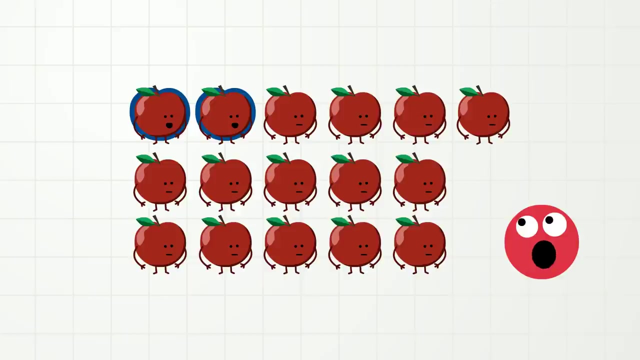 Seven. Okay, let's take a break and watch a movie. Okay, that's enough. Last one with even more apples, but this time no funny hats. Wow, so many apples. How many? Let's count One, two, three, four, five, six, seven, eight, nine, ten, eleven, twelve. 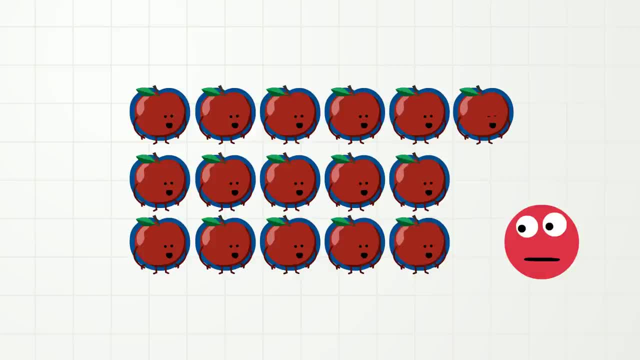 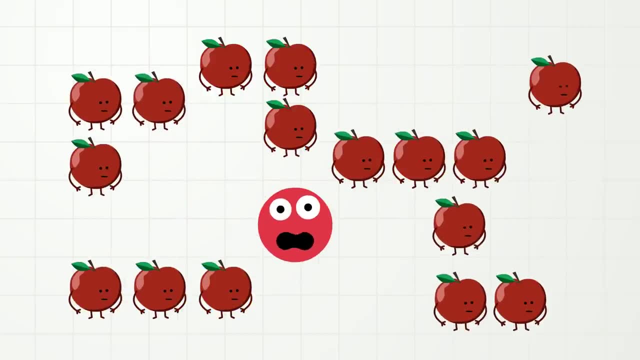 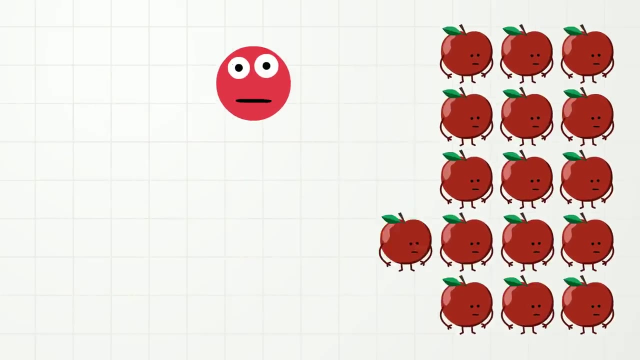 thirteen, fourteen, fifteen, sixteen apples, And there are many, many, many ways to compose or put together sixteen apples, and also to decompose or take apart the sixteen apples. Let's try some. Sometimes, when we are thinking about numbers, it can be easier to think about. 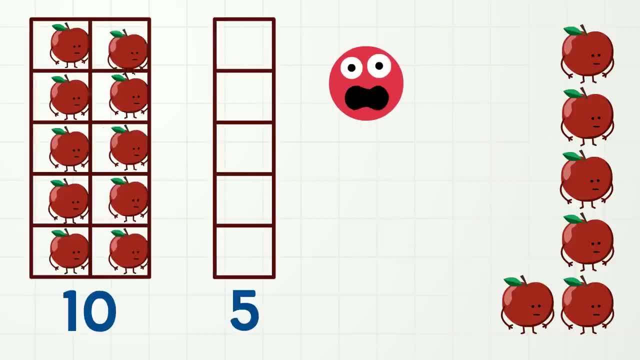 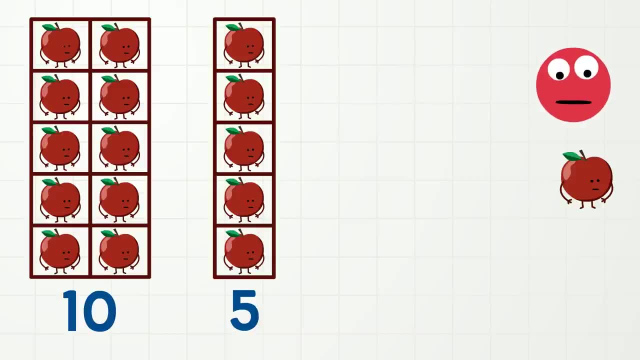 the numbers ten and five. So if ten apples go here and five apples go there, how many apples do we have left? That's right. one. Ten plus five plus one is 16.. So the number 16 can be made up of the numbers 10 and five and one. 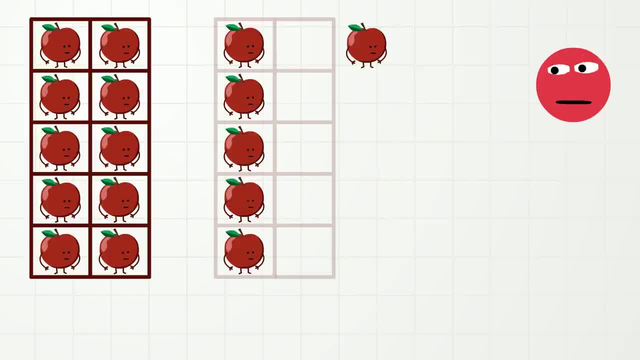 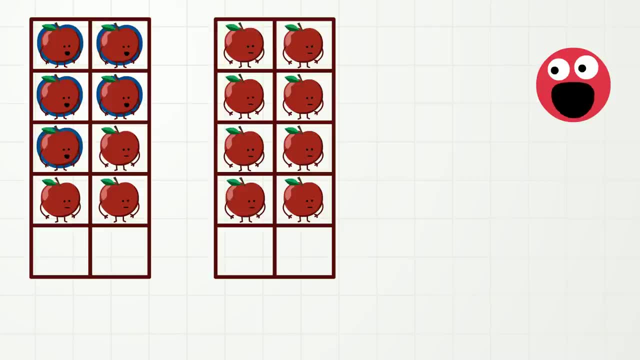 Cool, Let's try again. apples Move. Oh wow, now we have one, two, three, four, five, six, seven, eight apples over here and the same number of apples over there. Eight plus eight is 16.. 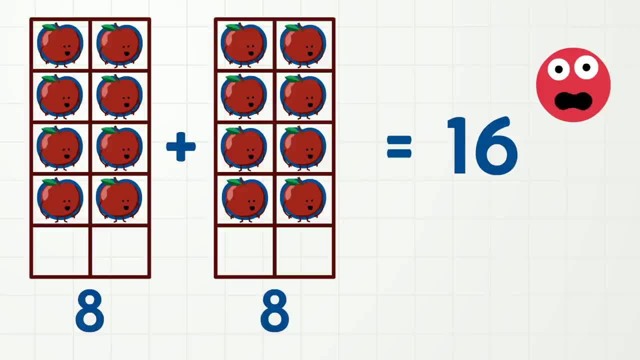 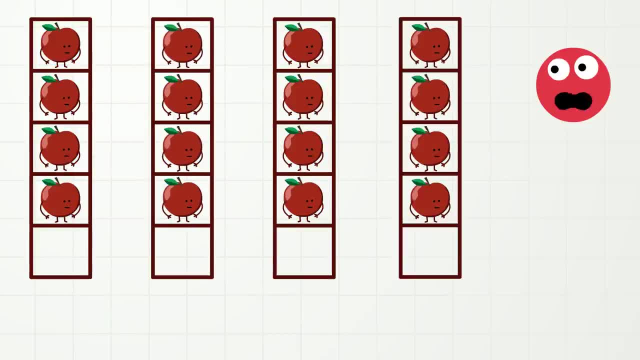 So the number 16 can also be made up of the numbers eight and eight. Okay, one last time. move apples. Oh cool, Now we have one, two, three, four, four apples here and the same number four apples here and the same number four apples here and the same number four apples here. 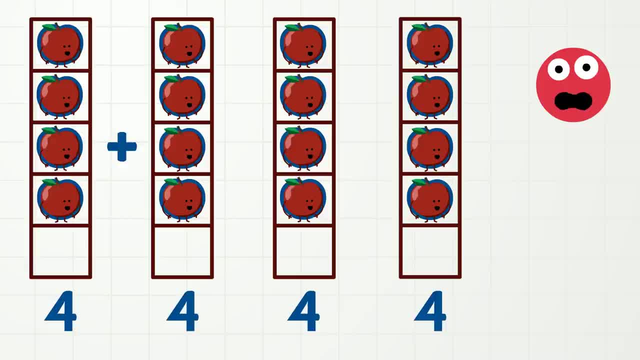 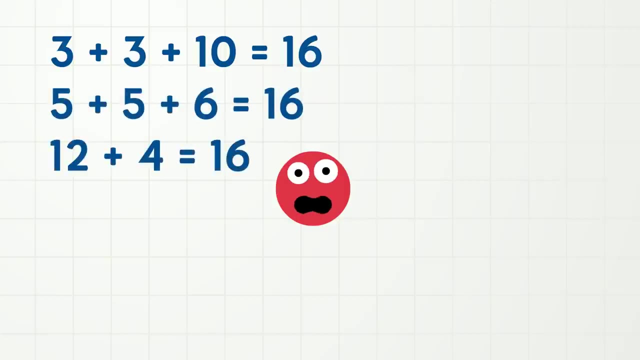 Four groups of four. Four plus four plus four plus four is 16.. So the number 16 can also be made up of the numbers four, four, four and four, And guess what? You can also make up and take apart the number 16 with other numbers that we haven't even practiced yet.